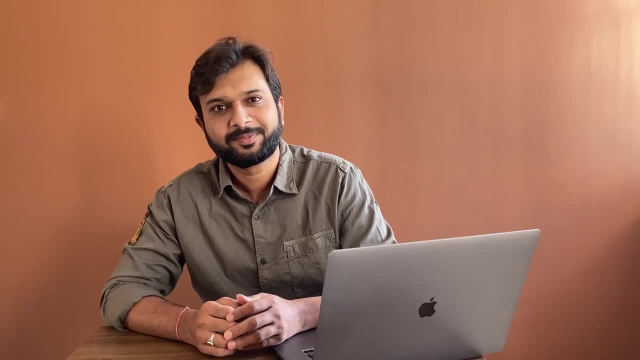 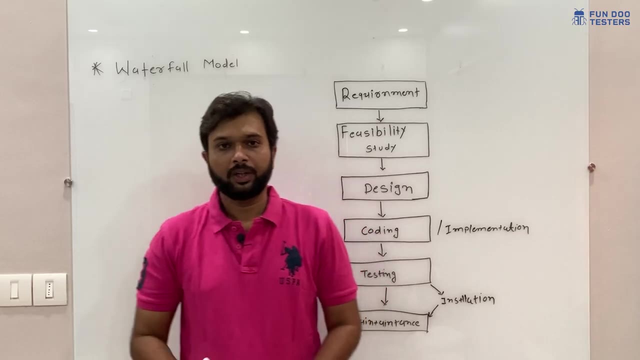 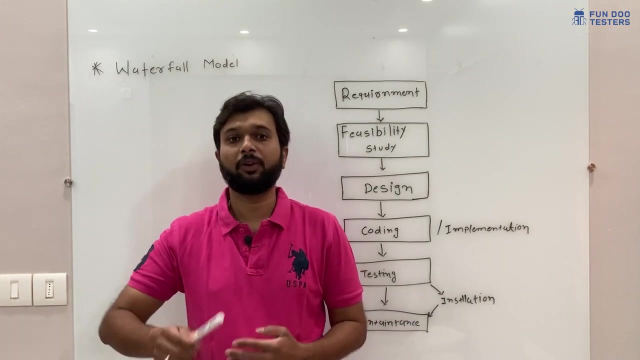 let's start after this small intro. In this video we are going to discuss what is a waterfall model, what is the advantages of waterfall model, what are the disadvantages, and when we are going to use the waterfall model. So this is simply how waterfall model looks. 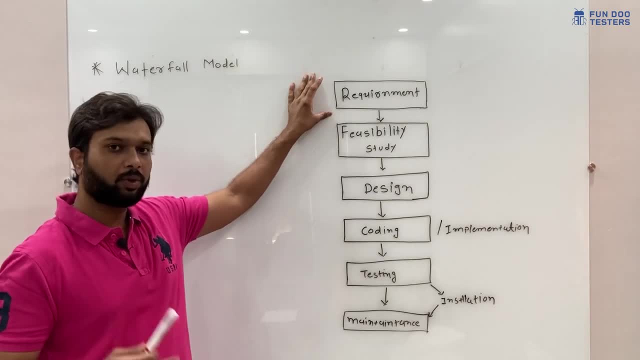 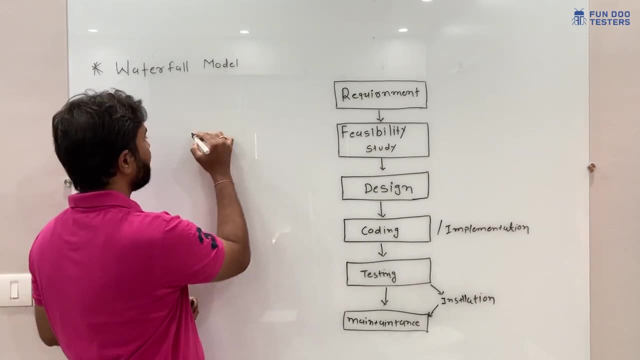 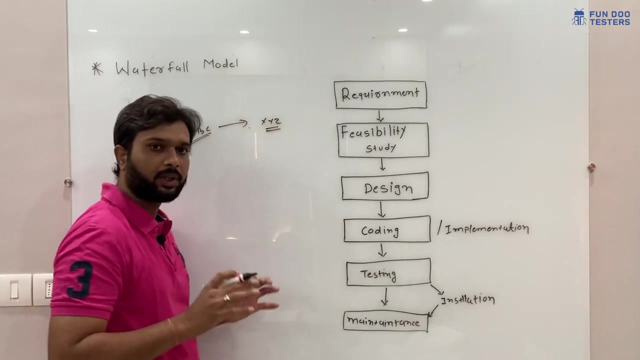 So initial stage is a requirement gathering. So in waterfall model, what will happen? when client is clear about the requirement, they come to the any company. For example, ABC is client and he is going to XYZ company. So by that time what they will do: client is clear about the. 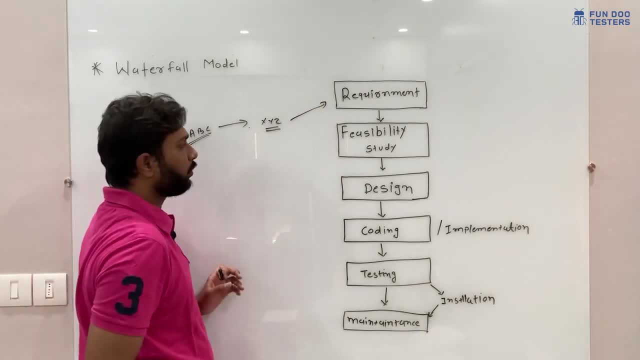 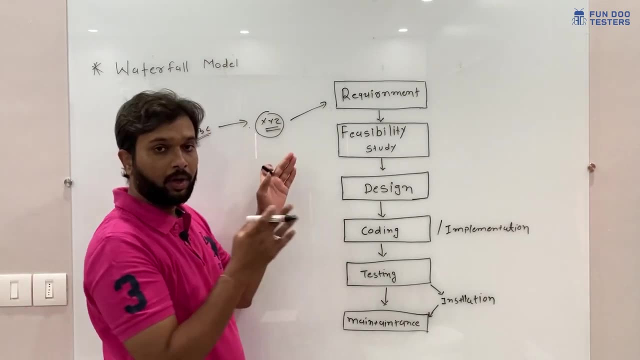 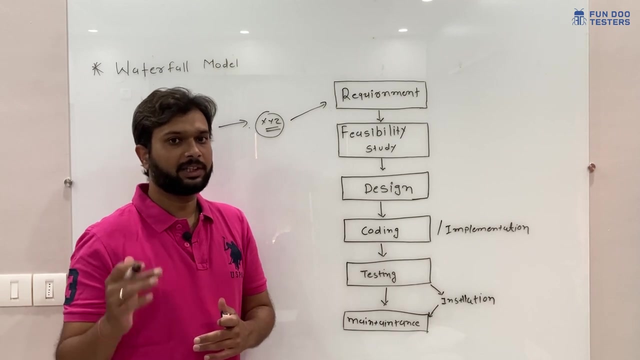 requirements. He will explain the requirement to the client XYZ and once requirement is ready, then it will go to the feasibility stage. So here the question is: once requirement is ready, so they have to freeze the requirement. There is no further change in the requirement. So that's why they are doing the feasibility study. What does 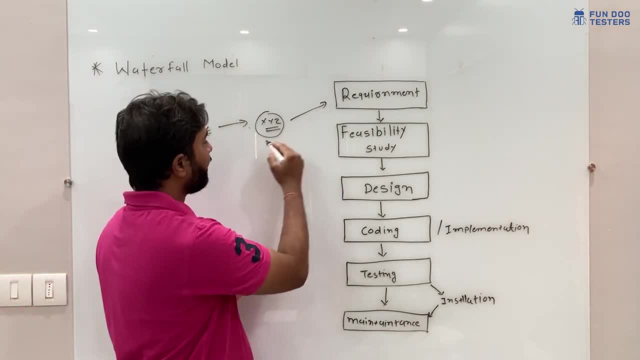 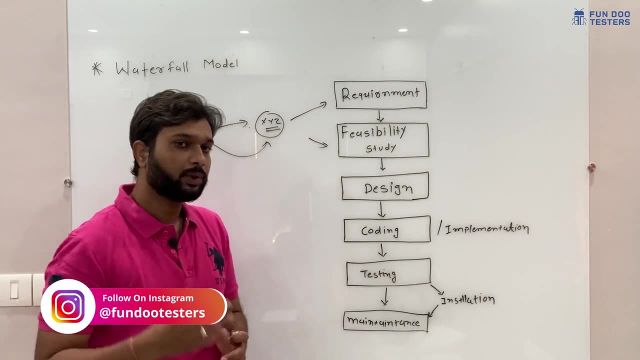 it mean In feasibility study they are going to make sure whatever client has come up with the requirement, that requirement they are able to implement using the code. So they are checking the feasibility And here there is no backward step. So if here it will fail, 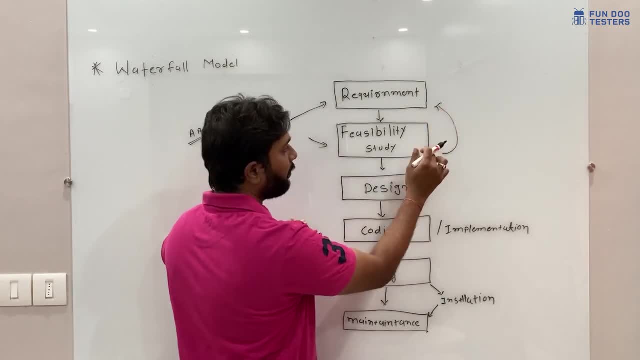 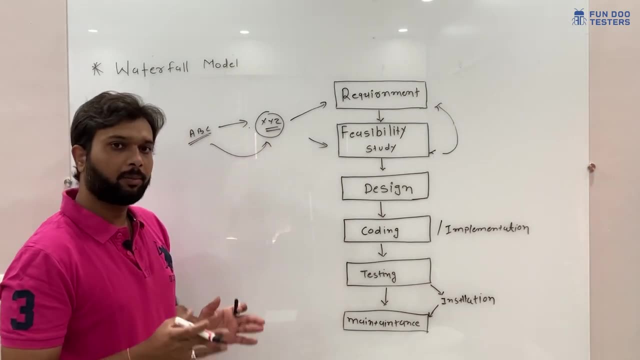 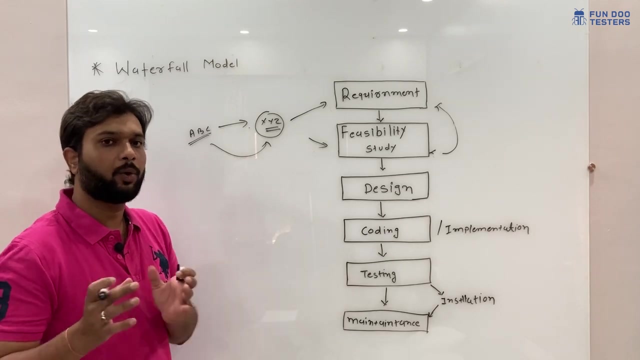 then they are not going to change here Because this is the principle of waterfall model. is saying: In waterfall model, when they are going to adopt, everything is concrete. There is a very less or 99%. there is no error chance. So by that time they are going with the waterfall model. Once feasibility study 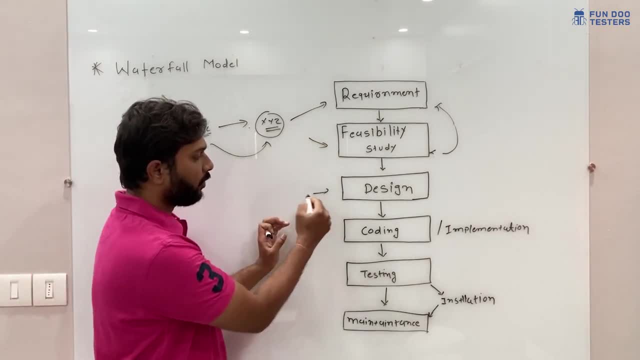 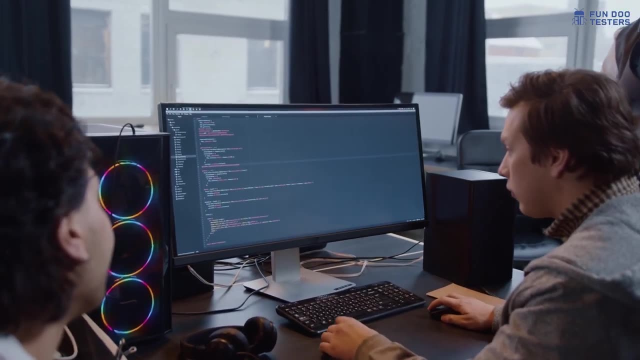 done. after that they are going with the design In design. they are going to create a proper design of the software and then it will go for. the coding Developer will start coding. Few people are saying implementation, or we can say coding as well. Later on it will be a testing, Otherwise we 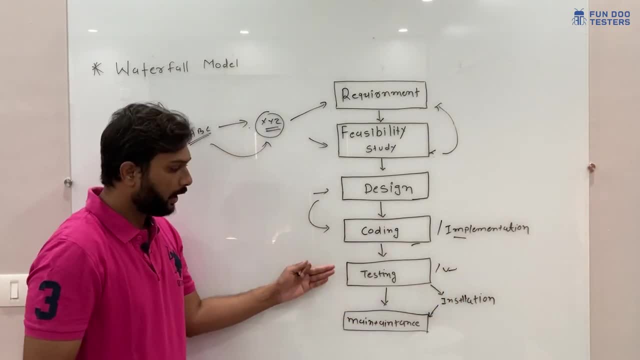 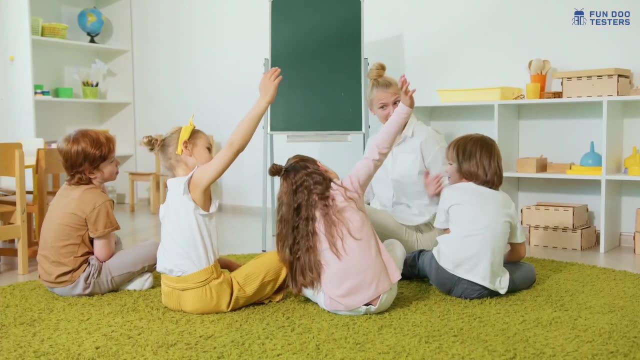 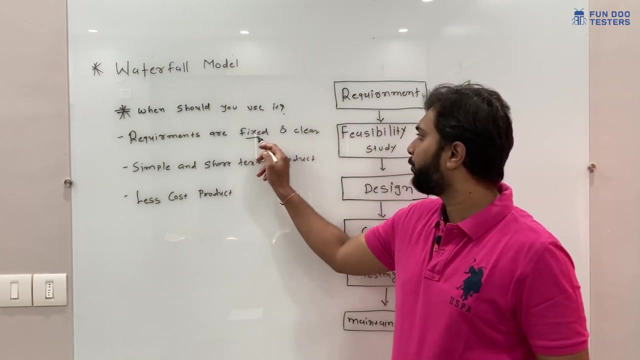 can say here: verification, And once testing is done, it will go for the. there is a small phase of installation and then maintenance. So this is how waterfall model works. So now question comes: when should we use waterfall model? So first is when requirement is fixed. 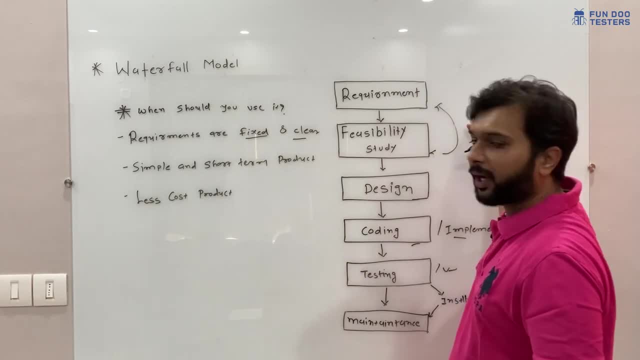 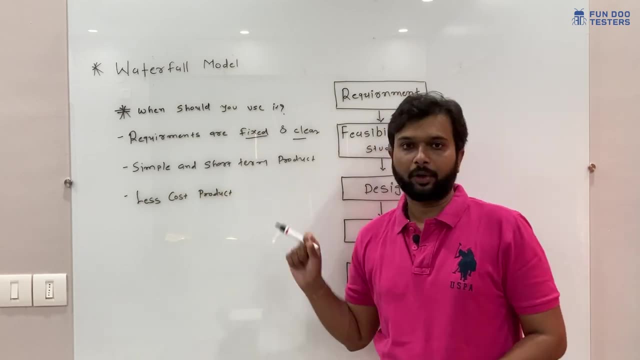 and clear, Because we are not going to back on previous stage. So that's why we need clear and fixed requirements. The next point is simple and short term product. So, for example, let's say we are working on a long term product. So, as of now, my current requirement: we have 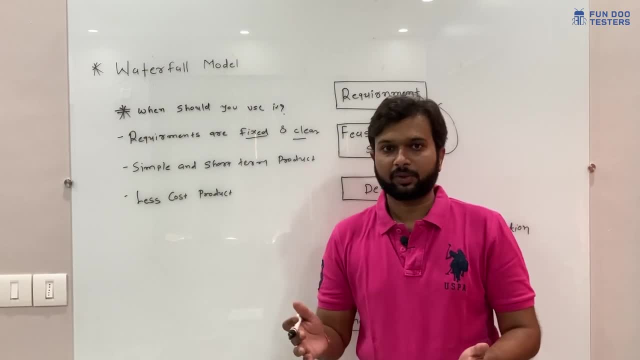 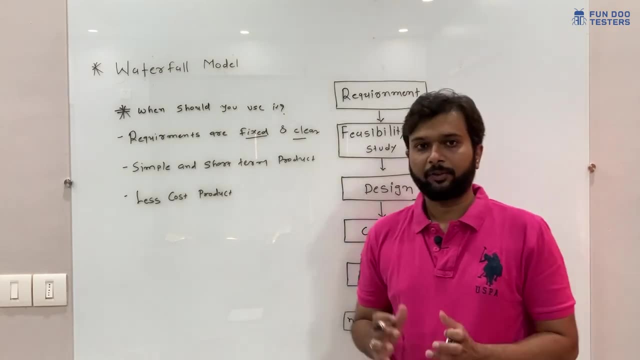 defined. So later on, after two years or three years, market is going to change. By that time we need to change the requirement. So this is the costly process in the waterfall model. So that's why whenever project or product is small, by that time we are going with the waterfall. 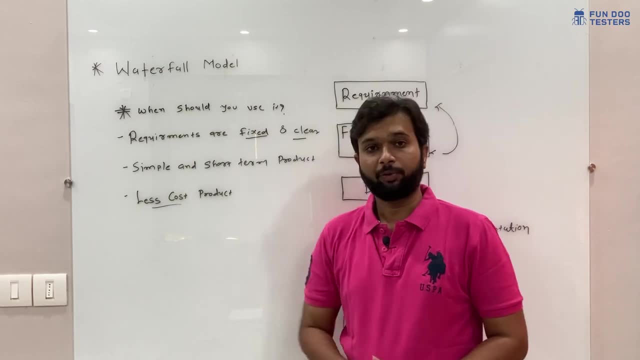 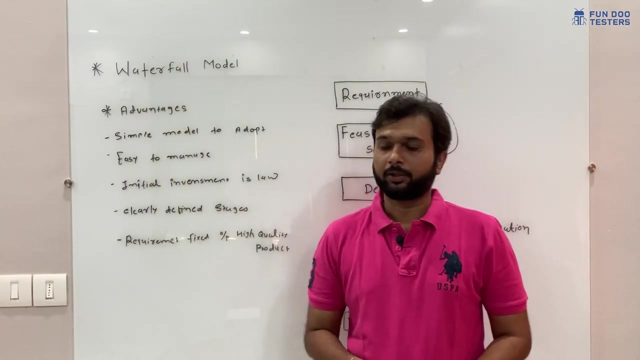 model. Now The third point is when the cost is less, Definitely when product is small, by that time cost is less. So in that case we will go for the waterfall model. So now let's discuss on the advantages of waterfall model. So first, 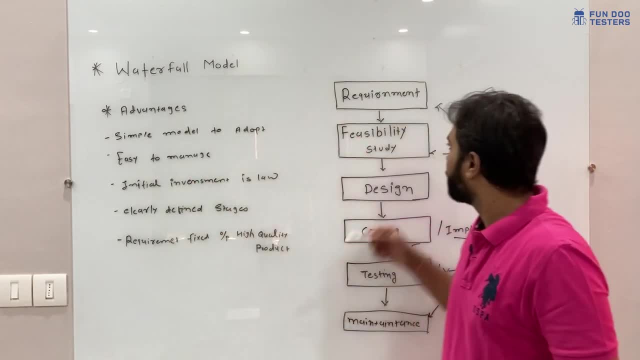 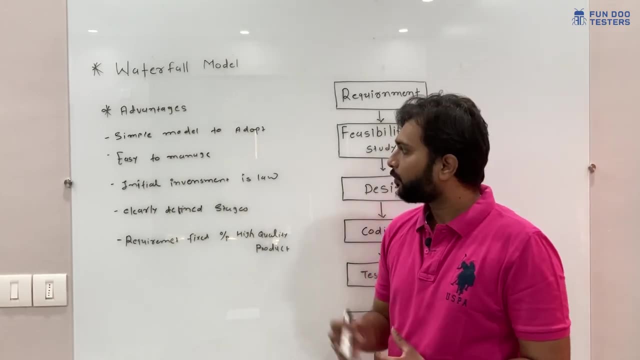 waterfall model is a simple model to adapt, Because this model has only these stages and we are not going back. So it is easy to manage and easy to adopt. Easy to manage. Another thing: initial investment is low. So this is the very important point. 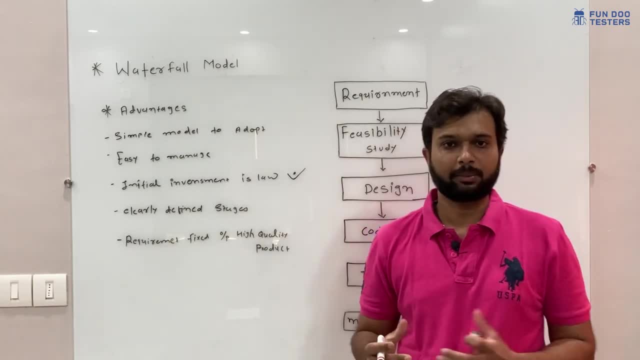 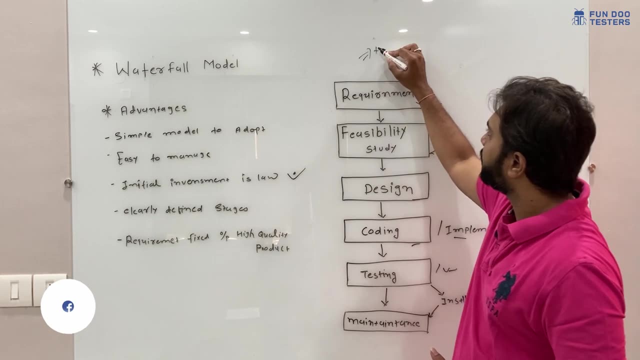 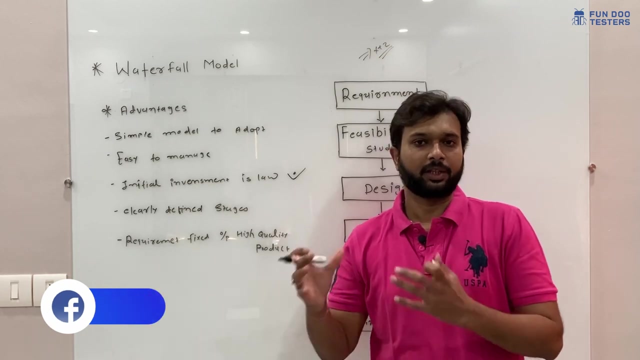 and port why initial investment is low. so, for example, i have one product idea and i want to build the product. so what i will do? i will go with the one company, which is xyz. so i will discuss initially, i only will discuss with the uh, their project manager, all sales team, xyz company. 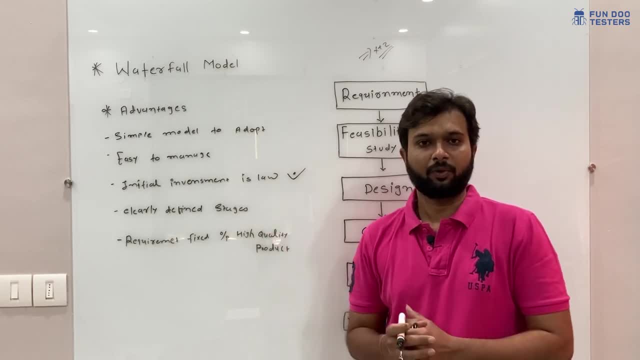 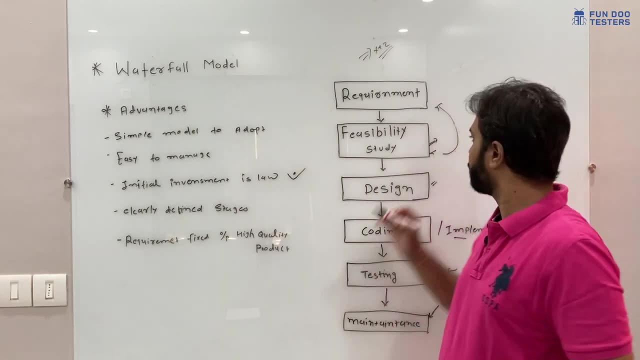 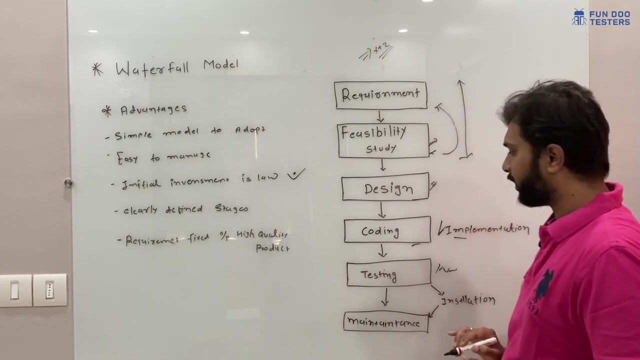 employees or project manager, all sales. they will understand the requirement and they will understand the project. later on, we will move to the feasibility stage and then design phase. so till now- this, when these two phases is complete- we don't need designer, code developers or testing team. so by that time, what? what i can understand? initial investment is low because i have to deal. 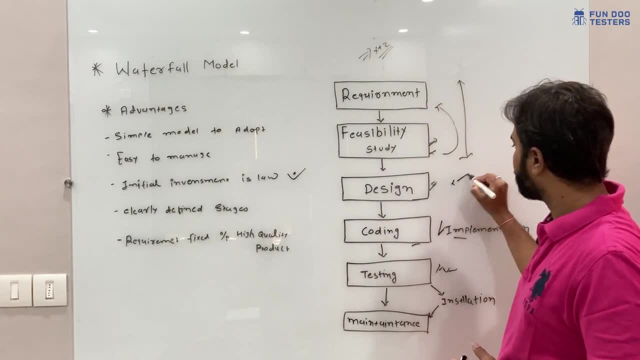 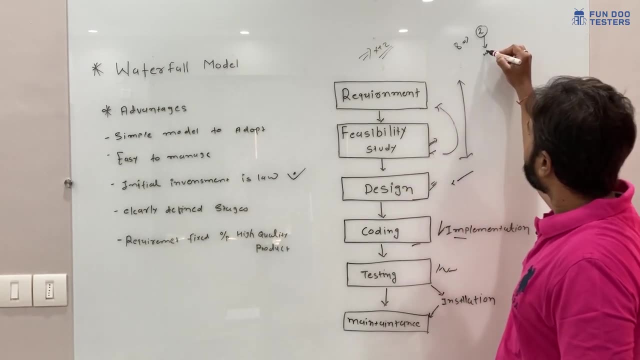 with only few people. later on i can hire, i can outsource the design for the few months. for example, project is around the eight months and i need designer for two weeks, only two weeks. so i can hire the designer for few times and then later on i will hire the development team for. 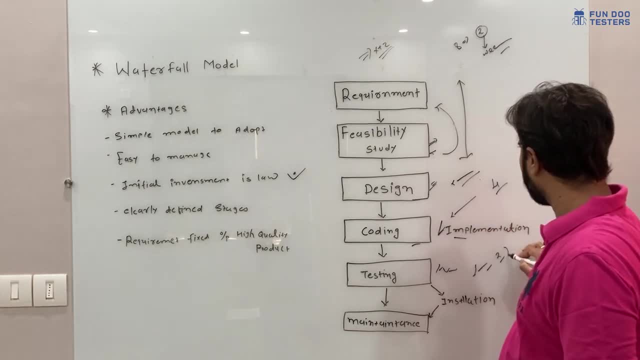 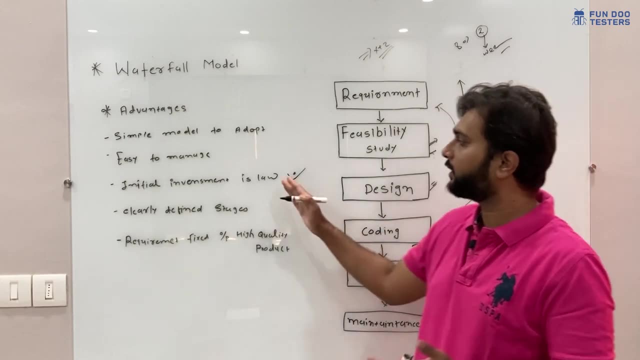 the- let's say, four months- and testing team, let's say for two months, because no one is going to work with any other people, because we need different person for the different stages. so that's why initial investment is low. and one more very important point is a clearly defined stages. 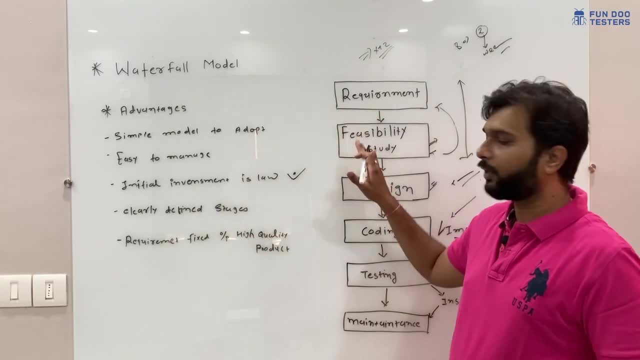 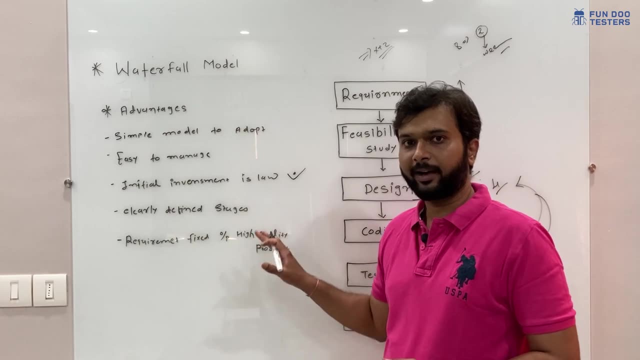 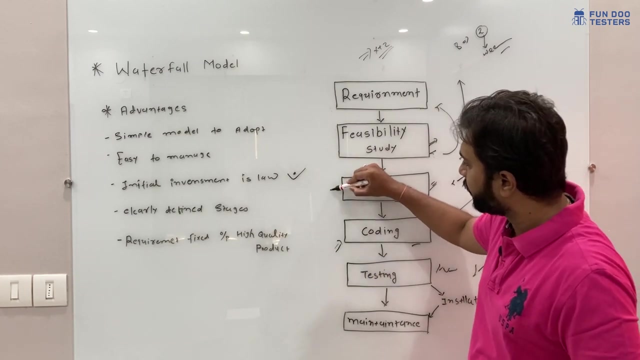 because what we have fixed requirement, we are not going to change the requirement on later phase. so that's what. everything is clearly defined and everything is clearly defined. that's why we will to change anything here. then again, this stage, this stage and this stage, we have to do the rework. but 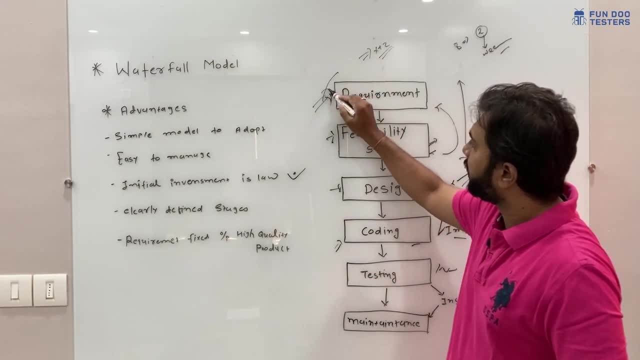 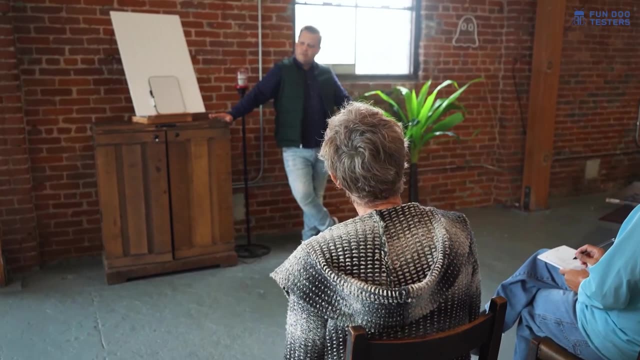 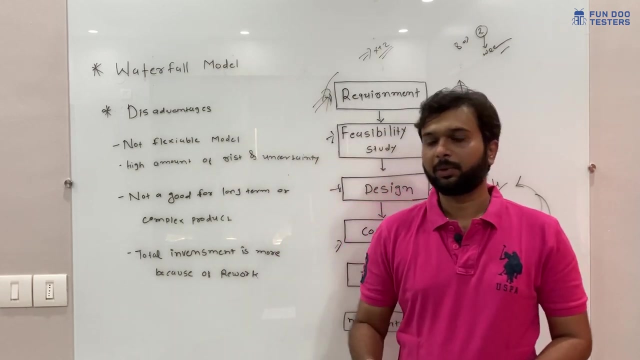 in this case we have this phase is clearly defined, so no need to do the further changes. so that's why this model will give high quality product. now we will understand the disadvantages of the waterfall model. so here this and this model is not a flexible model because we cannot change any. 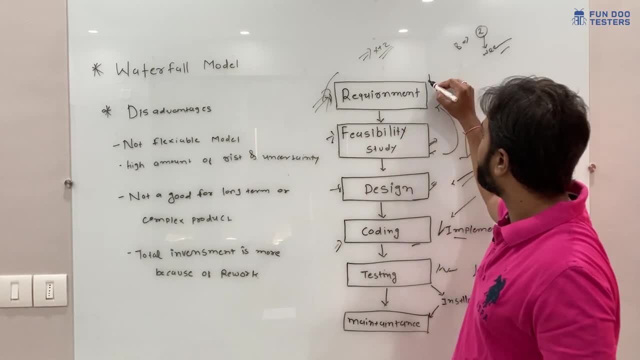 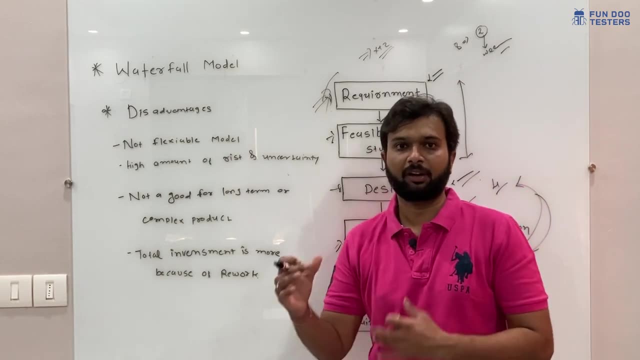 requirement or anything in any stages. once everything is freezed in requirement stage later on there is no changes. so in, for example, we are going to take for the long term project and after six months or one year we need to change anything because market is drastically changes in six months. 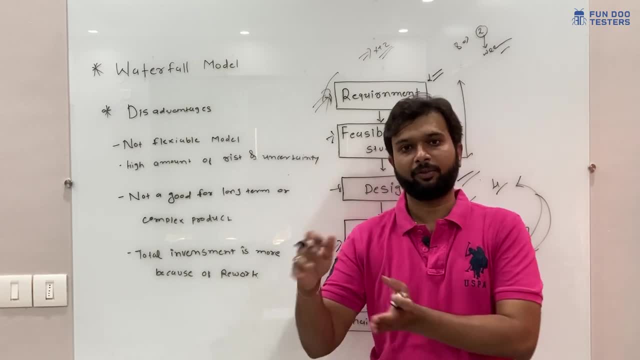 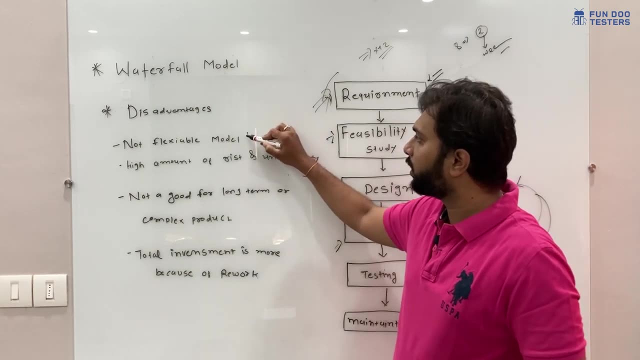 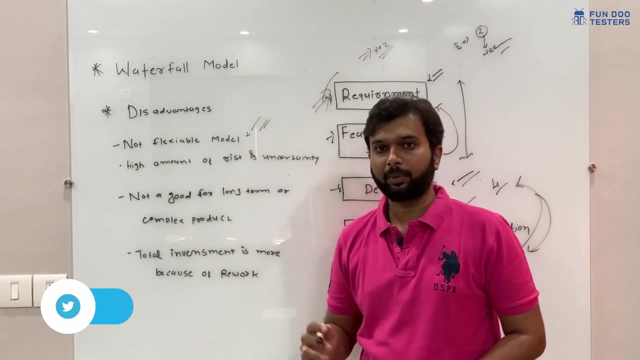 there are few applications available now. their application is outdated and we are moving on the new applications or new features. this is how industry work. so for this model is has very less capabilities later on, high amount of the risk, for example. if we want to change anything, then there. 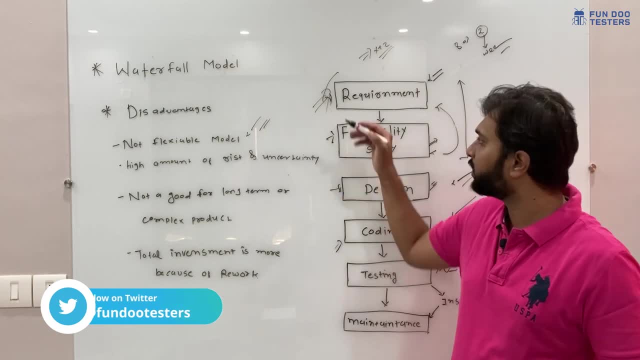 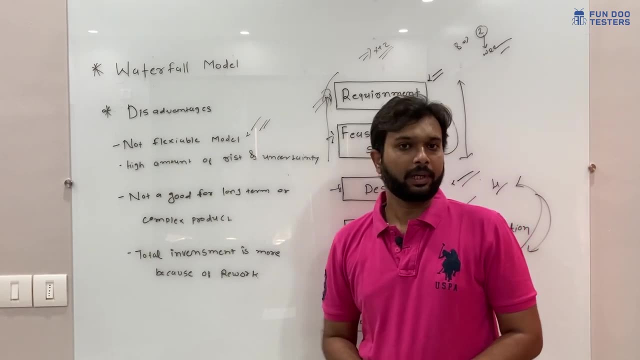 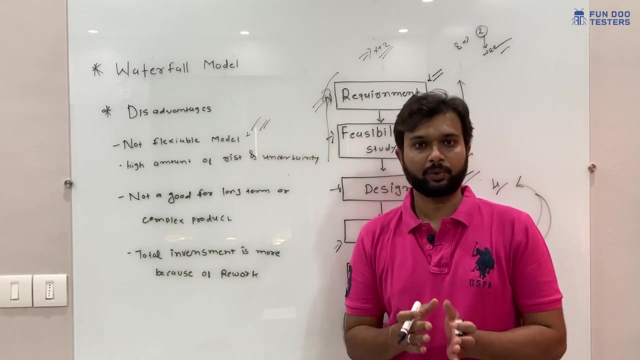 is a major risk because we we have to change many things in earlier phases. now this model is not a good for the complex or long-term product. why not good for the complex or long-term product? because, for example, from 2018 i have started one product, so now 2020, market will change, so 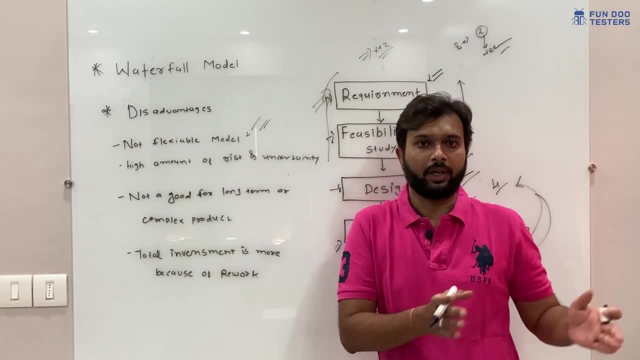 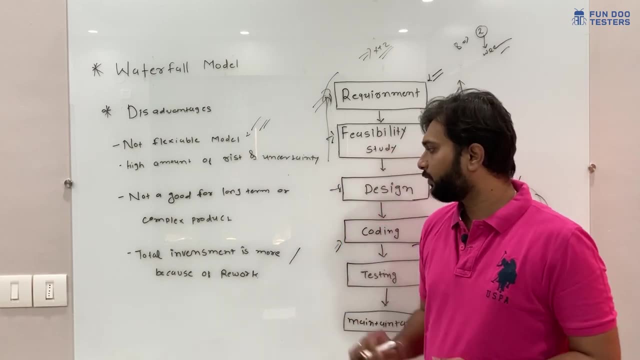 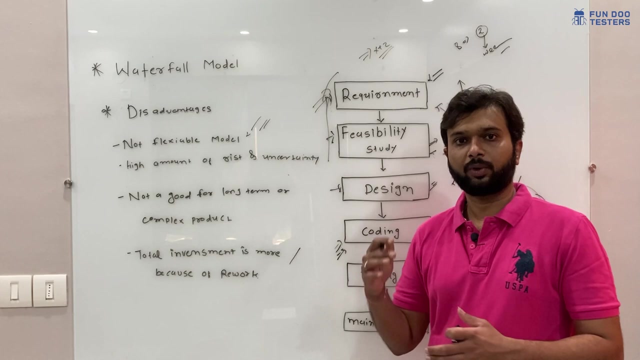 whatever i have started in 2018, it will go outdated. so that's why this product, this model, is not sufficient for the long term product and total investment is more because of the rework. this is why, if we are going to do the coding and it, it will take two years or we need to change anything due to some